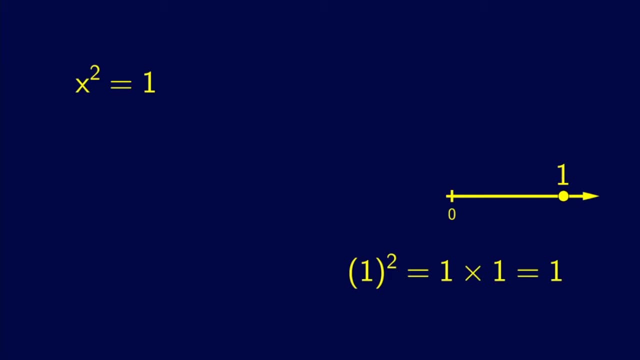 1 squared, that is, 1 times 1,, is still 1.. But most of you watching this likely know that there is a second solution. However, this second solution does not appear on the number line we have so far. In order to see it, we need to extend our number line to the. 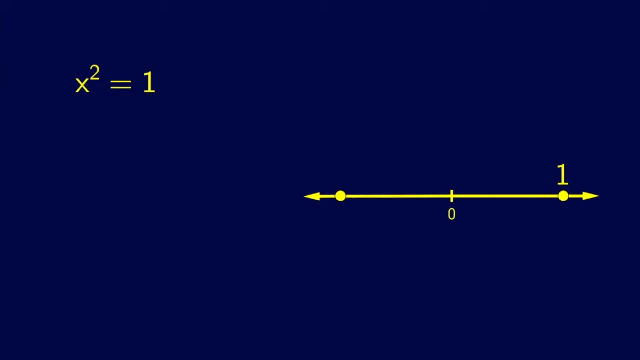 left of 0. These numbers have come to be called negative numbers. Our second solution is, of course, negative 1.. But why is negative 1 a solution? This may seem as silly a question. Most would just say because a negative times a negative is a positive and leave it at that. 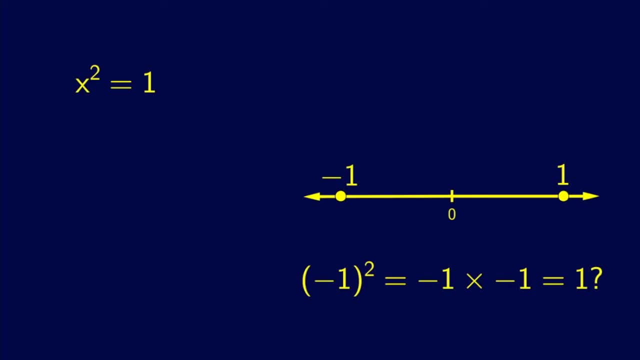 But again why. I don't want to just parrot some rule I learned in elementary school. We need to understand why negative 1 squared is positive if we are to extend this into higher powers. We know that negative 1 times 1 has to be negative 1.. That multiplying by 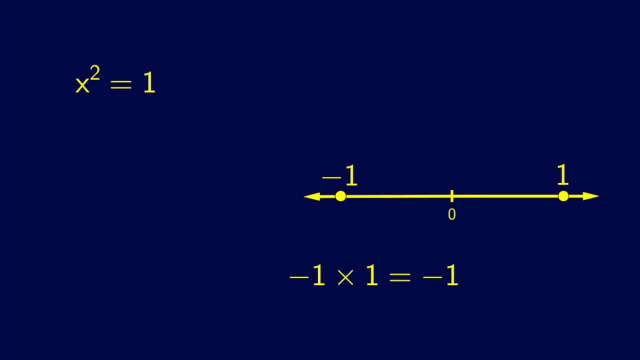 1 doesn't change. another factor, If you play wasoe and create a two-dimensional structure is a fundamental property of both 1 and multiplication that we would like to preserve. Another fundamental property of multiplication is commutivity. That is, 1 times negative. 1 should have the same result as negative 1 times 1.. 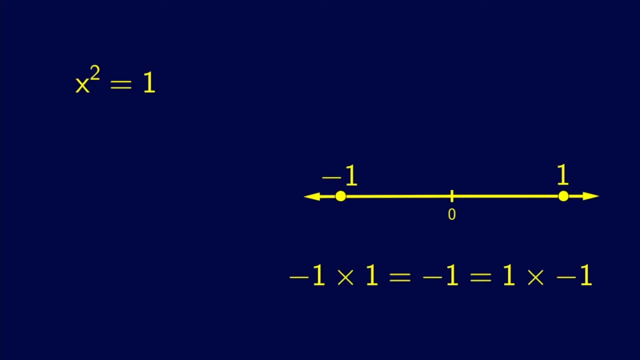 So 1 times negative 1 should be negative 1. if we want to be consistent- and mathematicians sure want things to be consistent- Let's look at what multiplying by negative 1 looks like geometrically. Multiplying by negative 1 keeps our distance from 0 the same. 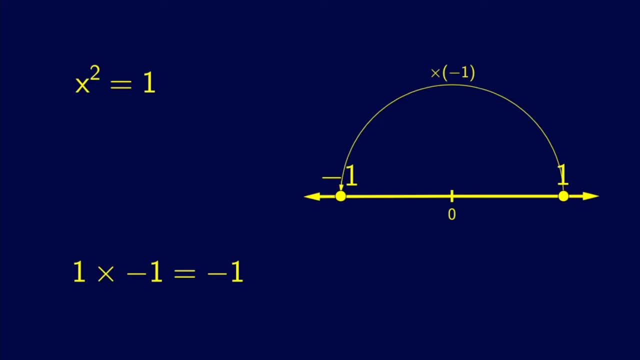 but rotates our position about 0. half a revolution Neat. So sticking with that, if we start at negative 1 and multiply by negative 1 again, we're back to 1.. Cool, You'll see shortly how useful this geometric view will be. 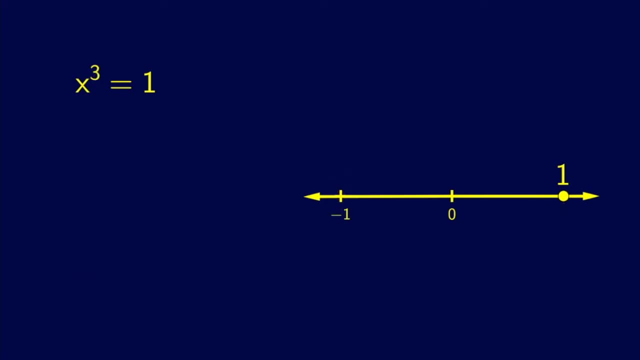 Alright, let's go to x. cubed equals 1.. Again, we have the obvious solution of 1, but why stop there? Indeed, the pattern established thus far would suggest that there are additional solutions here and here, all three solutions equally, spaced around this circle. 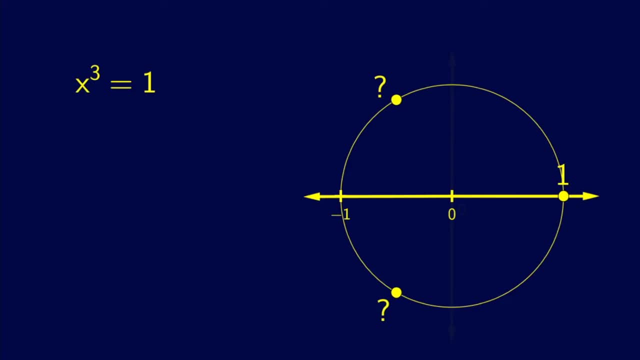 These solutions are clearly not on the number line we have thus far established. but that didn't stop us before, when we just extended the number line to the left of 0, and we've got plenty of additional directions to go. A sensible choice would be to move perpendicular to the line we already have. 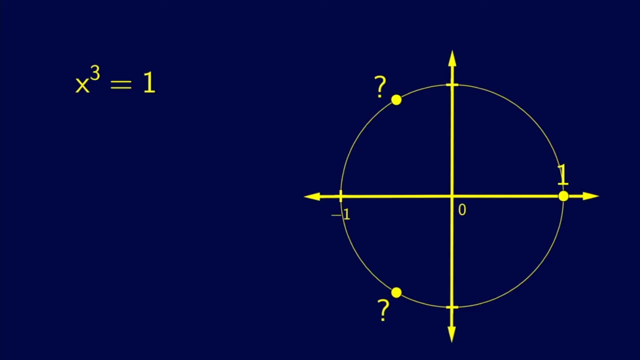 Just as negative numbers are different than positive numbers, the numbers along this axis are different again and require some symbol to denote them as such. Personally, I would have preferred continuing the pattern of a different symbol ahead of the digit, but what has become the convention is to use the letter i here. 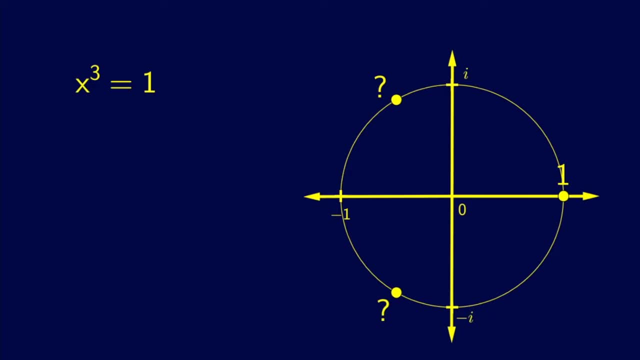 i, for you guessed it, the unfortunate word imaginary. We need to figure out some stuff about i. Well, i times 1 is clearly i, as would be 1 times i, Just as multiplying by negative 1 is represented geometrically. 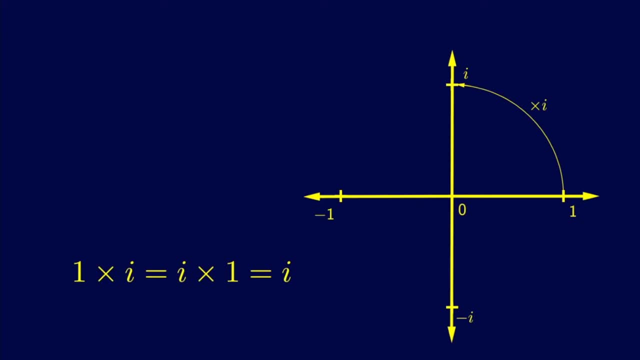 by a half-turn rotation. multiplying by i is a quarter-turn. This means that i times i or i squared is negative 1. Multiplying by i again gets negative i, which makes sense algebraically too, as i cubed, is i squared times i. 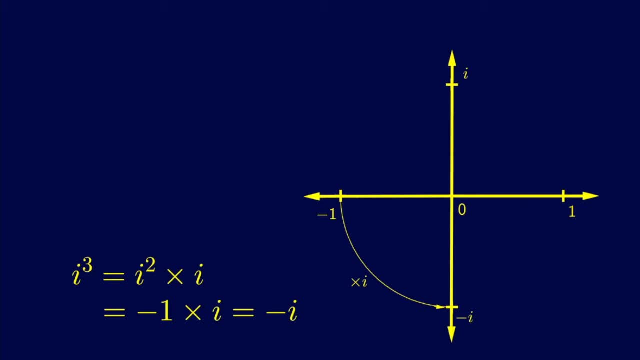 which is negative 1 times i, which is negative i. Finally, multiplying by i one more time gets us back to 1.. One more thing before we go: If i squared is negative 1, then it would make sense for i. 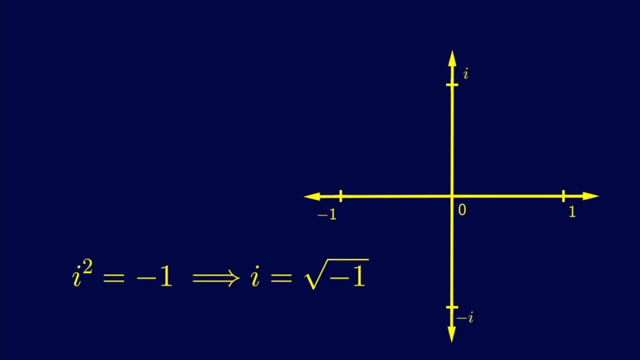 to be equivalent to the principal square root of negative 1.. Okay, back to our two missing solutions. It's actually pretty simple now to apply a little bit of trigonometry to see that these two solutions would be negative 1 half plus the square root of 3 over 2i. 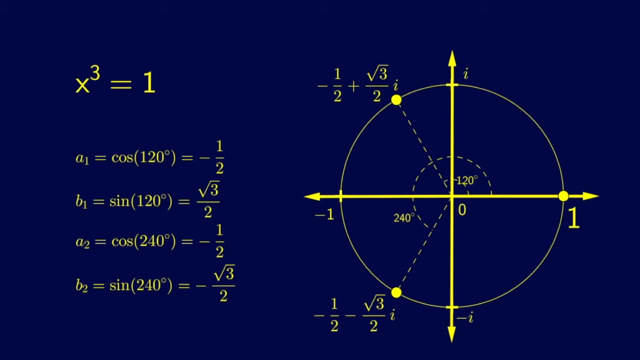 and negative 1 half minus the square root of 3 over 2i, Admittedly a bit awkward to say and by no means the only way to represent these numbers. it is important to realize that each of these points represents a single number. 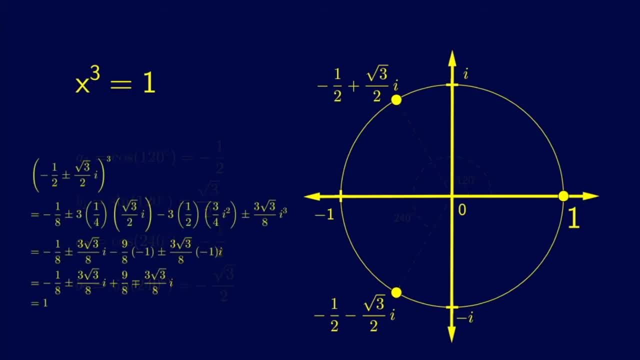 It's also easy to verify that these numbers are indeed solutions, with some basic algebra and remembering that i squared is negative 1.. And if you want, feel free to pause the video at this point to go over my algebra, There is now nothing stopping us from raising the exponent. 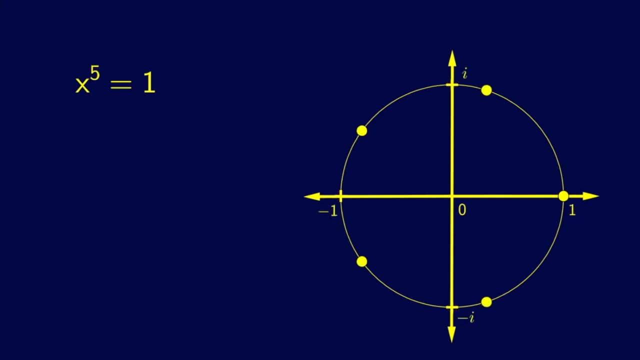 to whatever we want and expressing all possible solutions. It's also becoming clear that as long as we leave the right side of the equation, at 1,, all solutions are equally spaced around a circle of radius 1, centered at 0..